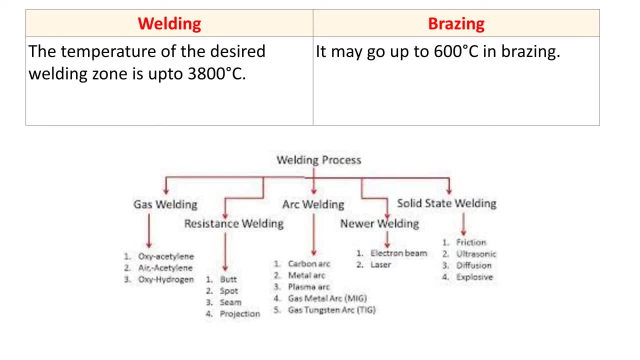 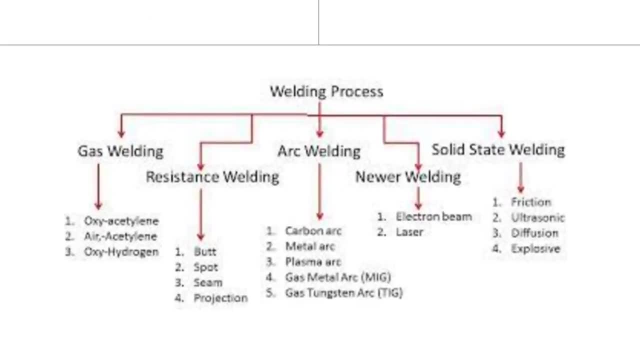 Celsius. So depending on the various welding processes, we get a different temperature during the welding. So here you can see the classification of various welding processes. So the welding process can be classified into gas welding, resistance welding, arc welding, some newer welding techniques. 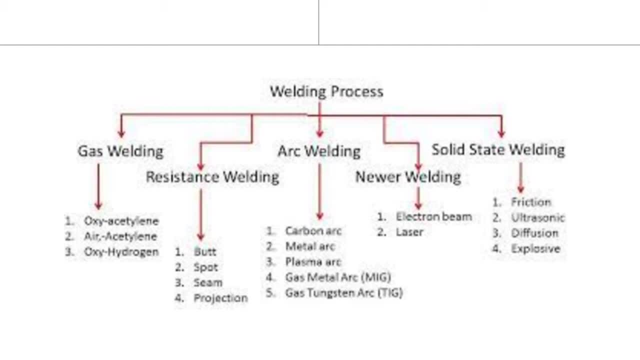 and solid state welding. We can further classify gas welding into oxyacetylene air acetylene oxyhydrogen. The resistance welding can be classified into butt spot seam projection, Whereas arc welding can be classified into carbon arc, metal arc, plasma arc. 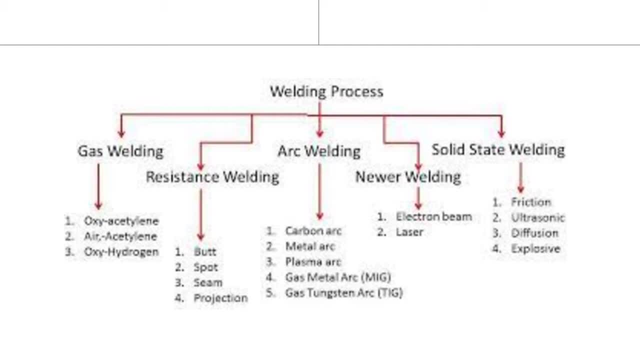 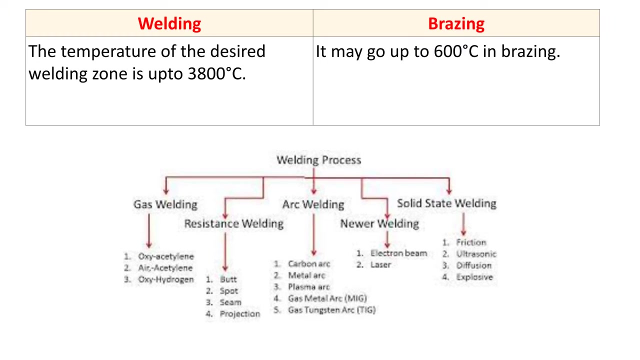 gas metal arc and gas tungsten arc. Few newer welding techniques are there, like electron beam welding, laser beam welding, And the solid state welding is classified into friction friction welding, ultrasonic welding, diffusion welding and explosive welding. So with this process we can achieve different temperature. Now brazing it may go up to 600. 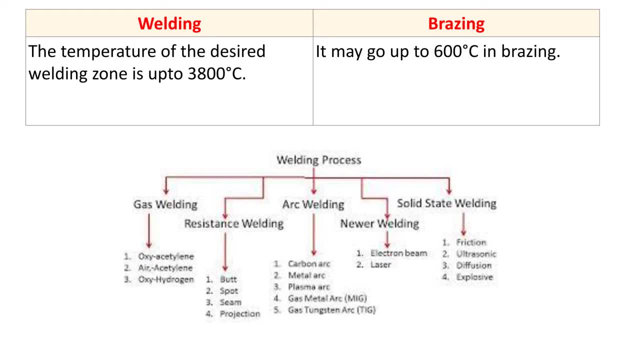 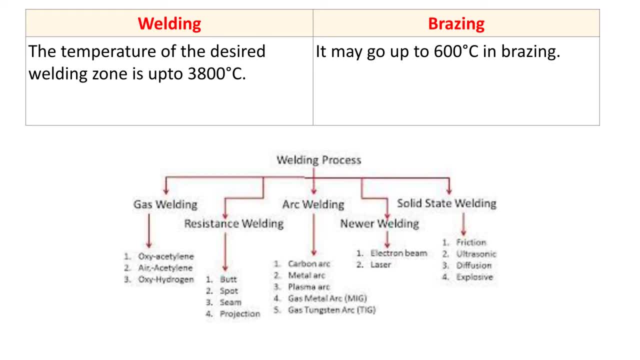 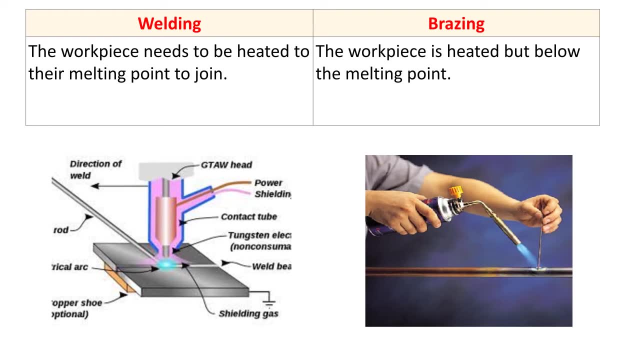 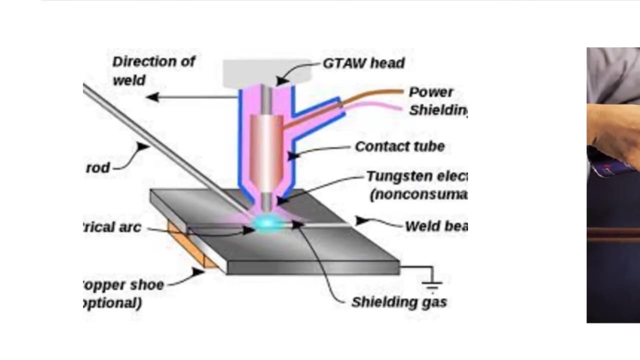 Celsius, Whereas in welding we can go up to 3800 degree Celsius. Next difference: the workpiece need to be heated to their melting point to join. So here you can see one of the type of welding process, that is, GTAW gas tungsten arc welding. 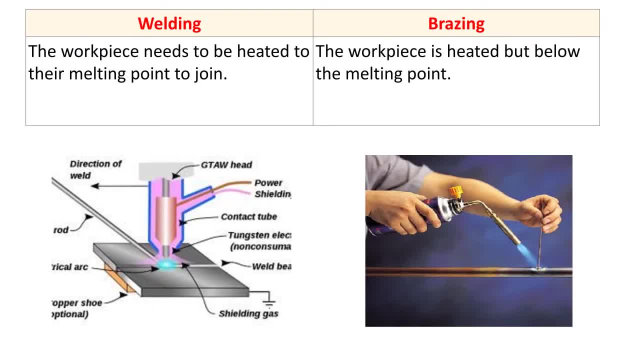 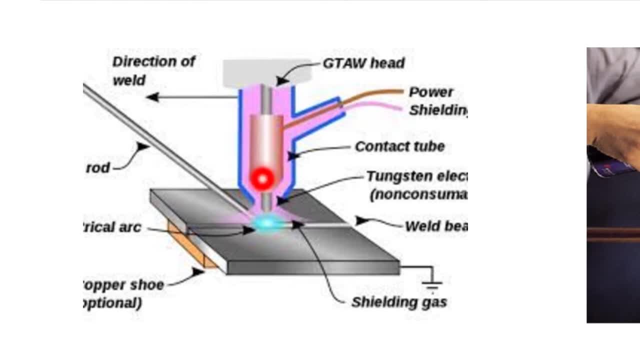 process. So in welding, what happens? we have to heat the workpiece above its melting point in order to join it. So this can be understand with this diagram. So this is nothing but a GTAW process, where we are using a non-consumable tungsten electrode. The arc is generated in. 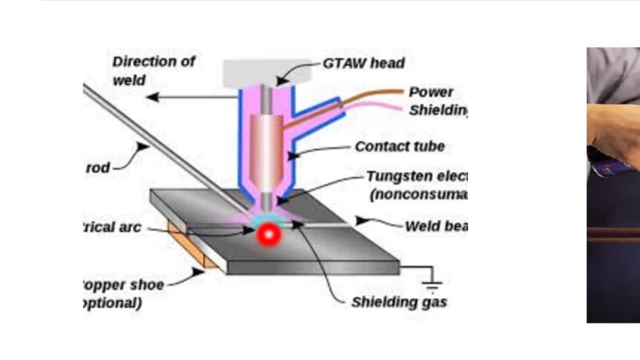 between this non-consumable electrode and the workpiece and due to that generation of arc, the heat is generated, and due to the generation of heat, the sing surfaces get melted forth and this gets the final flow of the work piece to be exhaust. Now let's see this for our 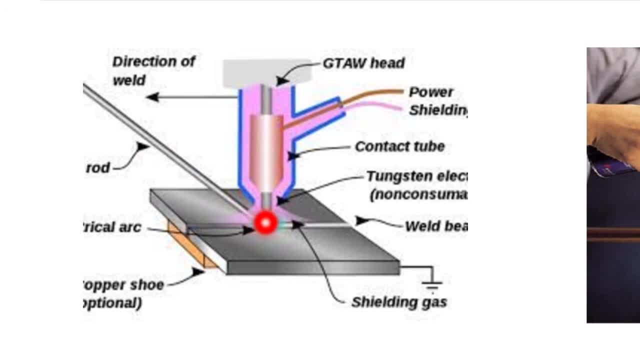 workpiece. What happens when you were the full in and out? And sometimes the filler material is in the form of an electronic base, but finished surfaces are receive some fluorescence from the worked piece and at the working base surface generate also used in order to join these two plates. so basically, in welding, what happens? we are melting. 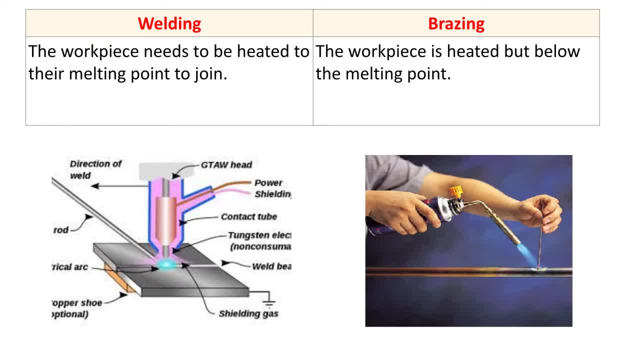 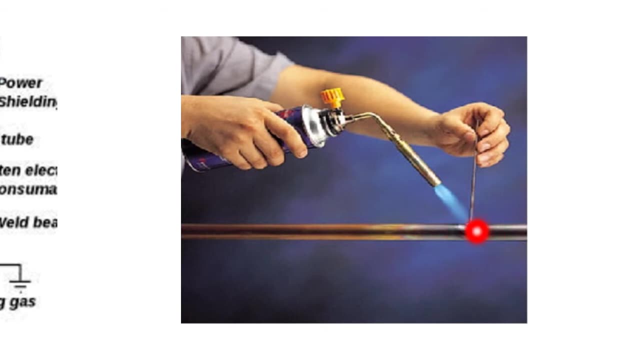 the parent material or the best material. so the workpiece need to be heated to their melting point. to join now the brazing: the workpiece is heated, but below the melting point. so here you can see the brazing operation. here also we are hitting the workpiece, but it is not heated above its melting. 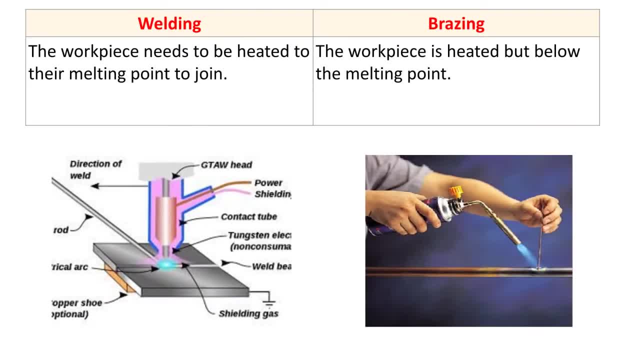 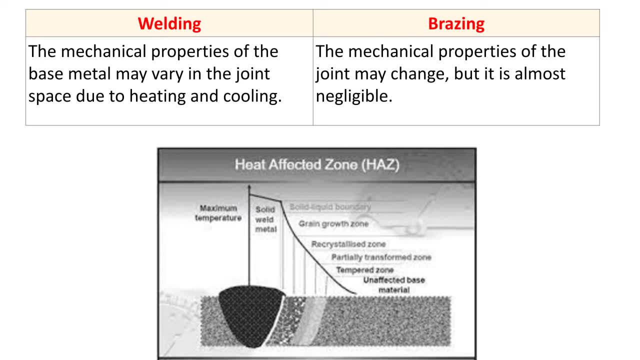 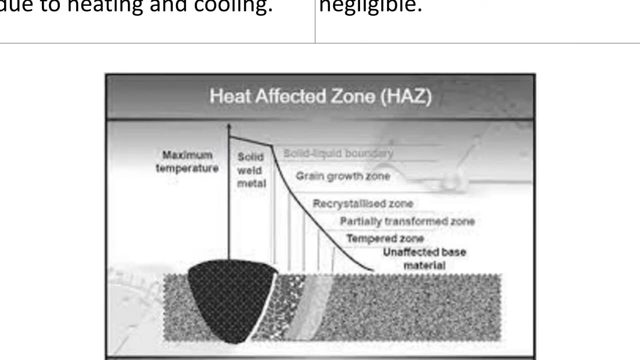 point. okay, it is heated, but below the melting point that is known as brazing. now, next difference: the mechanical properties of the base metal may vary in the joint space due to heating and cooling. this can be understand with this diagram. so here you can see the heat affected. 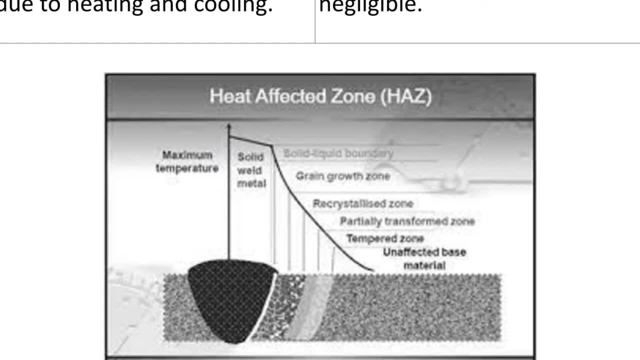 zone of the weld metal. okay, so this is nothing but the weld bead. this, the portion in black color, this is the weld bead and this is the heat affected zone. so this is the heat affected zone and this is the base metal. so here you can see the 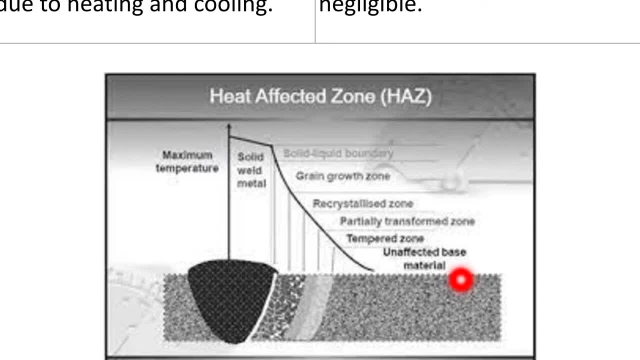 microstructure of the base metal is is different than the microstructure of weld bead and the heat affected zone again. we can classify heat affected zone in few few zones, like the solid liquid boundary, then grain growth zone, then the recalcified zone, then partially transport zone. 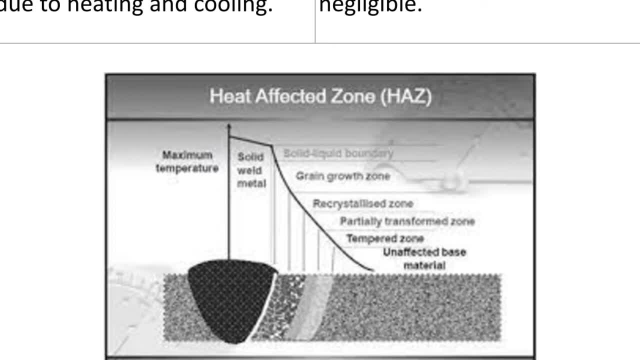 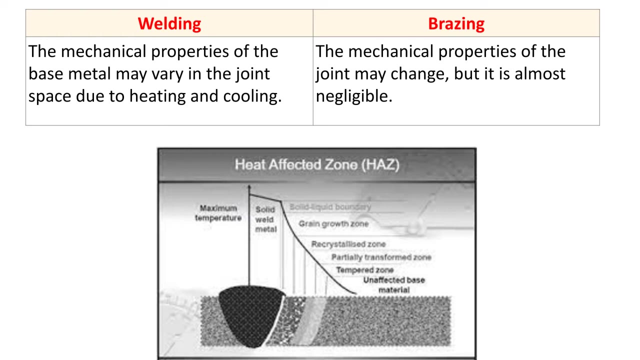 tempered zone and unaffected base. okay, this is base metal. so here you can see, the microstructure of the base metal is comparatively different than the microstructure of this weld bead and heat affected zone. so what happens as the microstructure changes? there is a difference in mechanical properties. okay, so the mechanical properties. 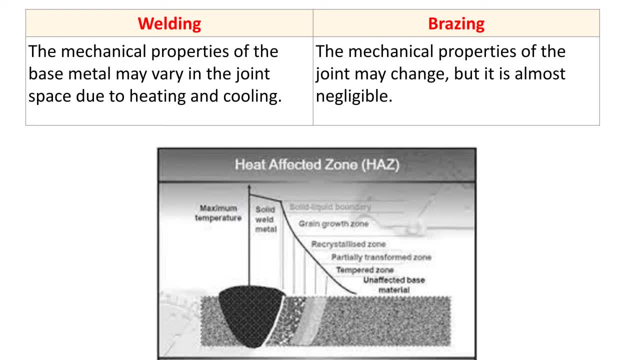 of the base metal may vary in the joint space due to heating and cooling. now brazing the mechanical properties of the joint may change but it is almost negligible. now in brazing what happens. we are heating the metal up to 600 degree celsius only so there is negligible change in the 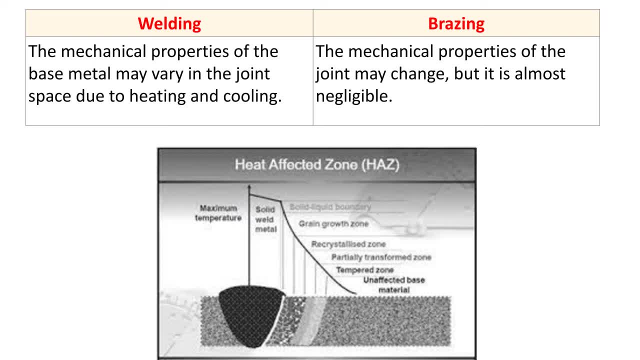 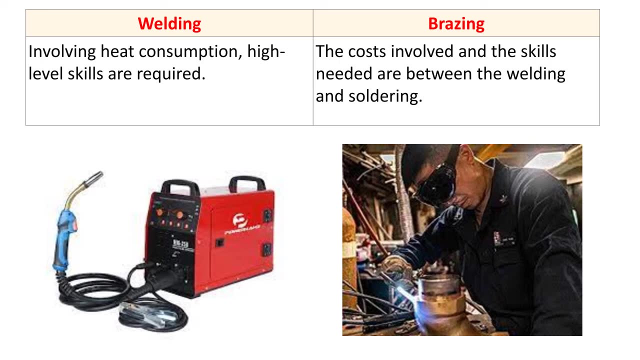 mechanical properties of the metal, whereas there is appreciable change in the mechanical properties of the metal in welding, because here we are heating and cooling. now next difference: welding involving heat consumption, high level skill are required. so here you can see the welding machine. so the welding is nothing but heat addition to the workpiece. so we are adding, we are adding.